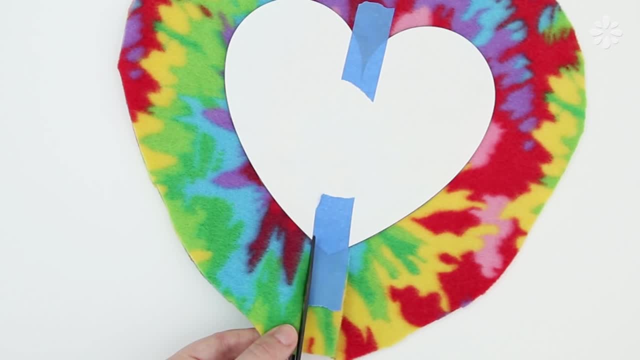 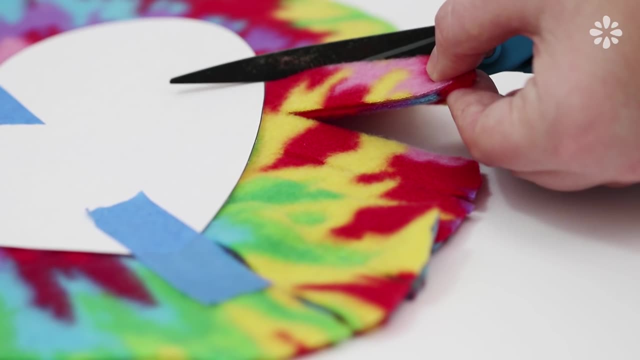 wide strips around the entire template, So you start at the edge and then end the cut at the template. These strips do not have to be cut perfect either, and you can use your thumb to estimate the amount of width While you're going, make sure you cut through both sides of the fleece. 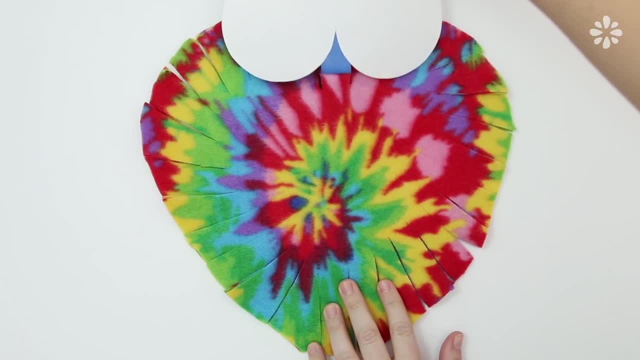 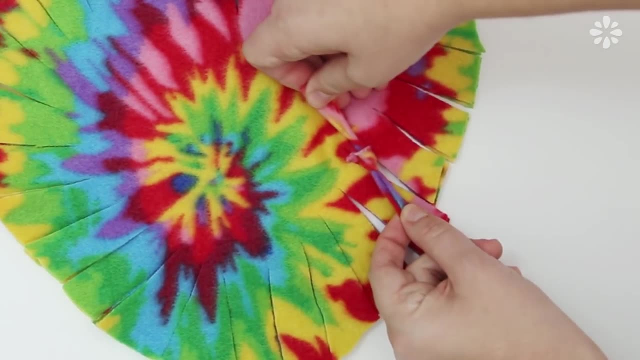 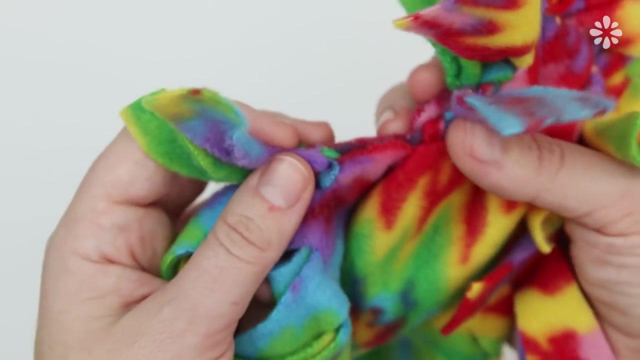 After you've cut strips all around the heart, you can then remove the template and start tying the top and bottom strips together in a knot, And make sure you leave a few strips untied so we can use that space to fill it up. If you have some areas between knots that are just too wide and you're 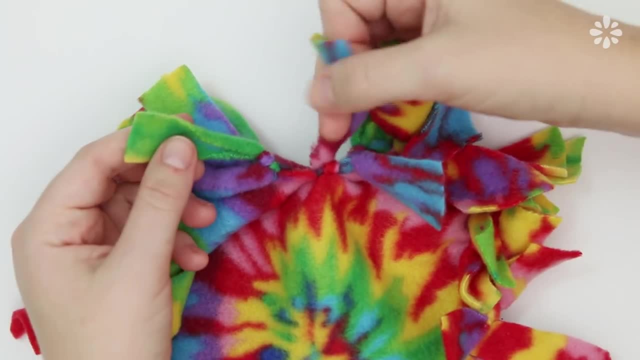 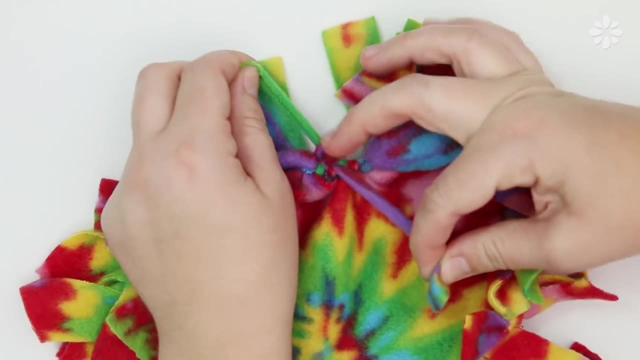 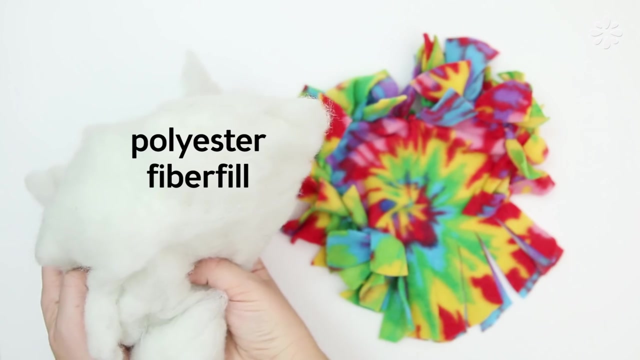 afraid that the filling will come out. you can simply take the strips from those two knots and then make another knot in between. So that will cover the gap and hopefully allow your toy to last a little bit longer Before your dog destroys it. Now, with a few strips left to tie, we can fill the heart toy I'm using. 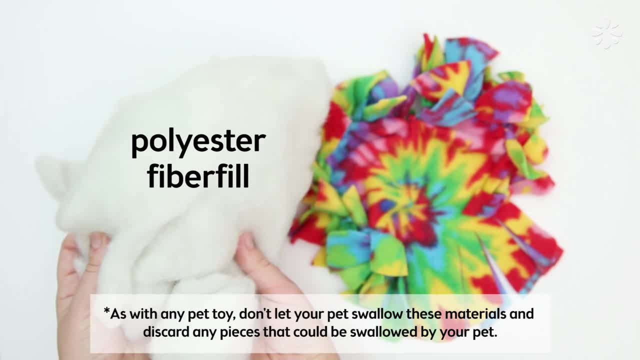 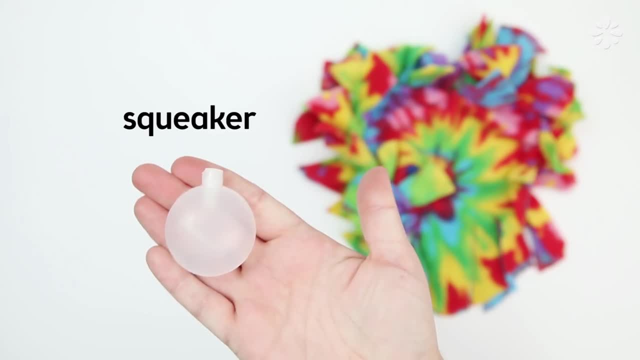 polyester fiber fill for this, which you can find at the fabric store or recycle from certain items, and I'm also going to add a squeaker into this which I got from one of Kona's destroyed toys. Add the filling in to the heart toy and I'm going to add the squeaker in the center. 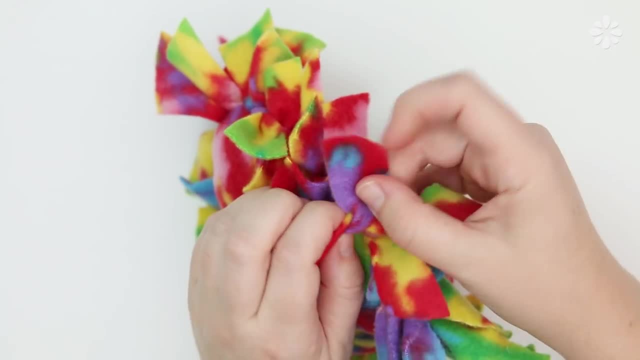 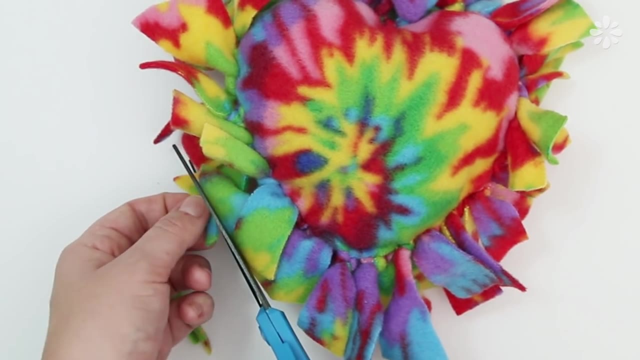 and then add some fill on top of that. Then tie the remaining strips into knots. The strips will be at different lengths, so you can go ahead and cut the strips so that there's an even border around the heart shape. And now this heart toy is complete and ready for the pup. 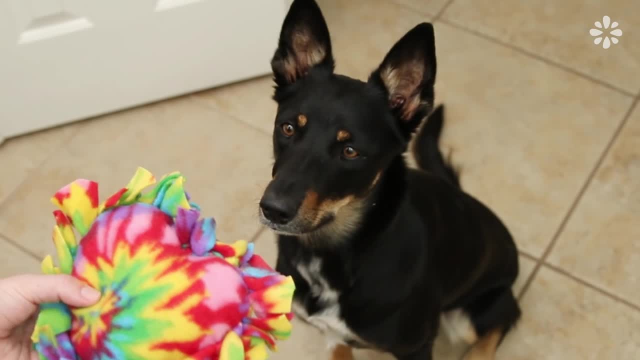 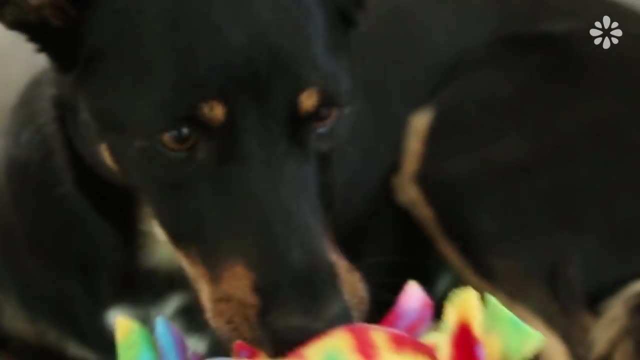 The whole time I was making this, Kona was sitting next to my work table waiting for me to be done with this toy. She just knew it was for her, And when she wasn't playing with it she was kind of using it as a pillow and giving me this: look like: yeah, get your own heart toy, this one is mine. 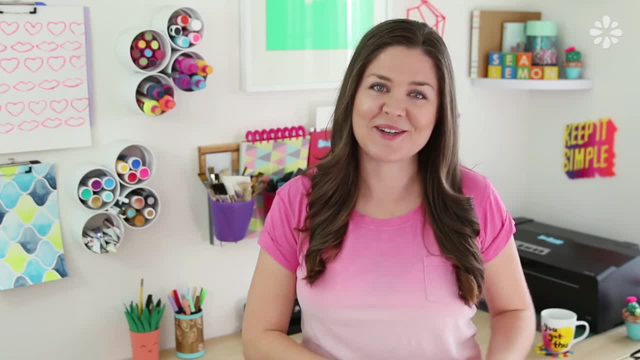 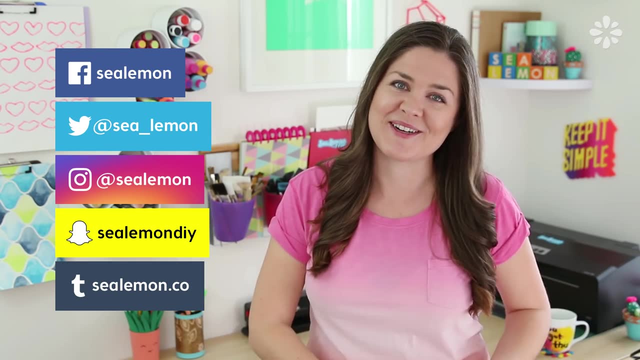 If you try this out, I would totally love to see pictures of your dogs and the toys, so share those with me on my social links. I'm a huge dog lover, so I would just love to see pictures of your dogs and, in a comment below, tell me what you love most about your dogs or pets. I would love to read about it and be sure. 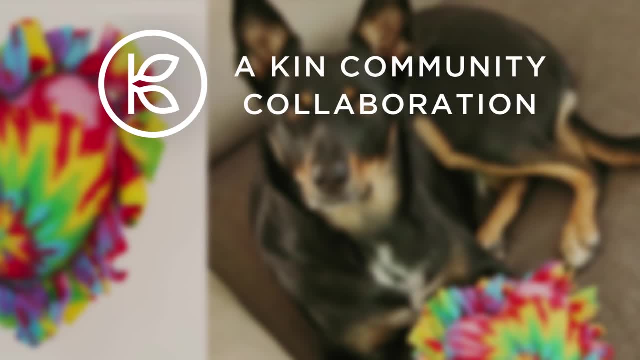 to subscribe to my channel, Sea Lemon, so you don't miss any of my videos. and don't forget to check out the rest of the videos in this playlist. Happy Valentine's Day and I will see you guys next time.